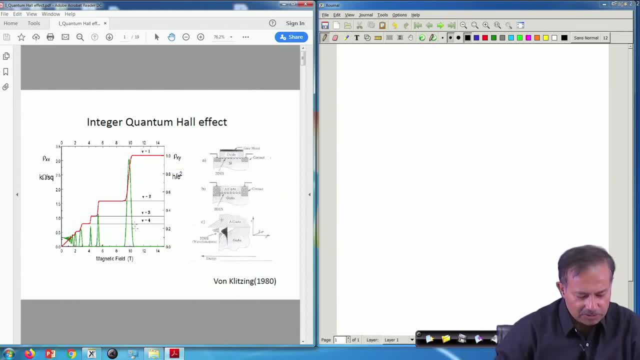 And at that point rho xx, which is the diagonal conductivity. the diagonal resistivity also jumps, but in the, during the plateau, the diagonal resistivity remains 0.. Now this plot is, with respect to rho xx, in kilo ohm per square, remember, in two dimension, if you remember your R equal. 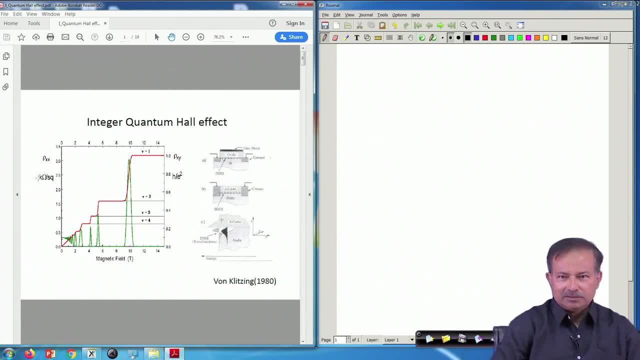 to rho L by a, Then you will find that A, which is the area, and L have The area and L have, So the area and L have the number of the plates. so this will be the protocol for the size of the plate. The area and the number of the plate will come Now, at that point. 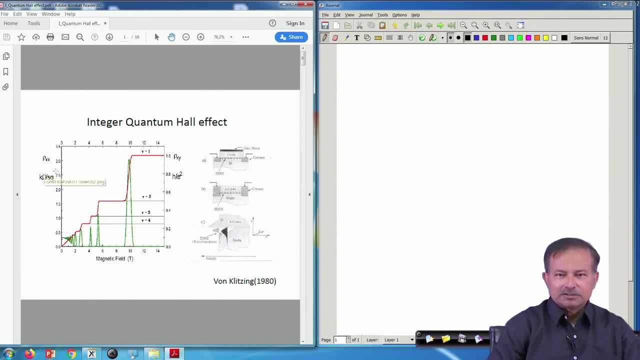 have the same dimension. So there this becomes a independent of the area and kilo ohm per square is the. So resistance and resistivity have the same dimension. So it is generally expressed in terms of kilo ohm, but kilo ohm per square area, So in two dimension that 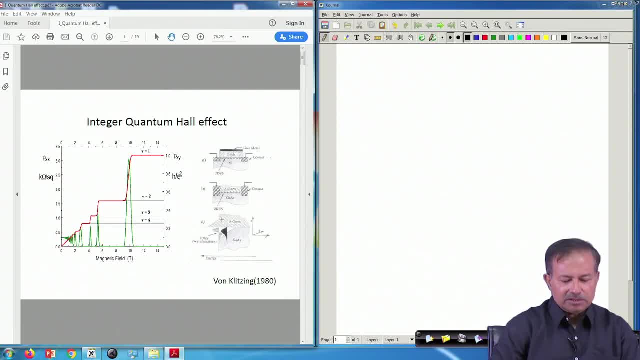 is the convention, Whereas this rho xy, as I will show later, has an, has a dimension as a, and it can be expressed in terms of two fundamental constants: which is h by e square, And so the rho xy is expressed in this unit and these nu? s are the values of the. 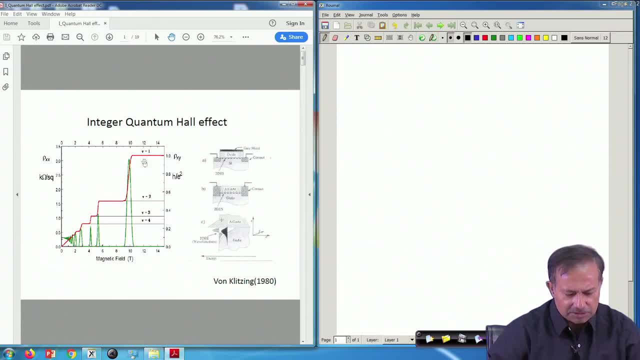 and these nu? s are the values of the, the values of the, the quantization in see, these are the numbers, number density of the Landau levels, which I will again discuss. But basically, what you have to look at now is that there are these plateaus which are extraordinarily quantized. I mean that is. 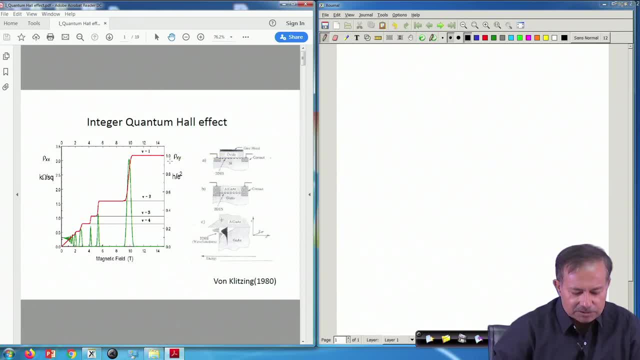 the real. look at the rho xy value. it is exactly 1 here and this value is really. So if you plot sigma xy, for example, this will be 1, this will be 2, this will be 3, and so on. 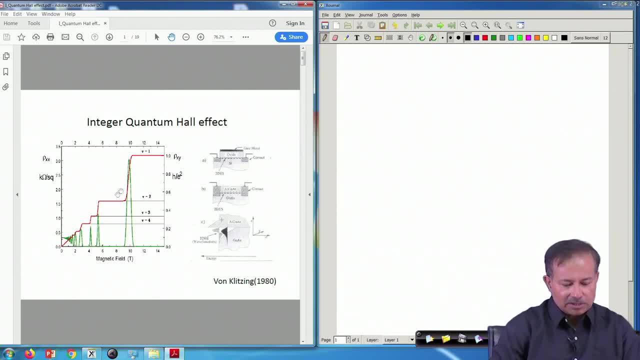 So these values- 1 here in rho, xy, 1 half and so on, these are quantized to almost few parts in billion. So these numbers are not approximate numbers. So that is where the surprise was, because if you remember resistivity, 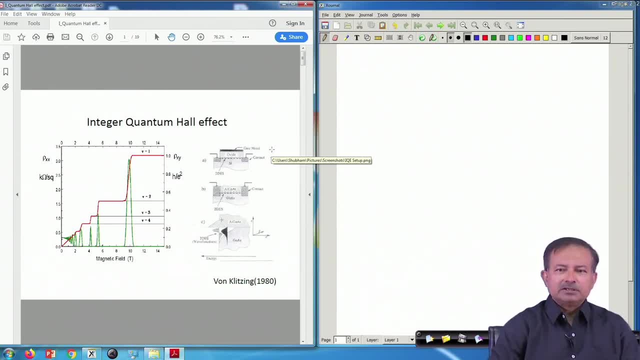 Resistivity is the property of a, of a material, and the material can have defects, can have impurities, can have any other things. In fact, if you keep the same material exposed to air for 2 days, you will see that your measurement of resistivity has changed, Whereas here, 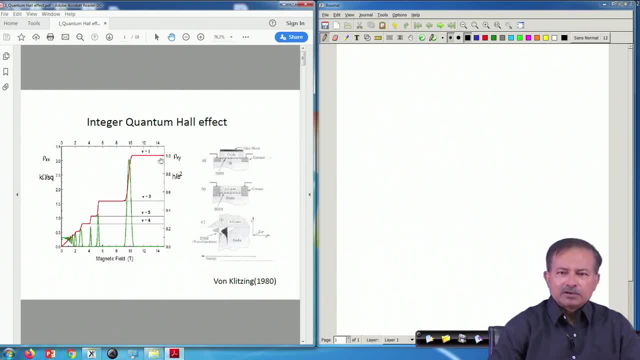 the value of this soft diagonal resistance or resistivity is extraordinarily fixed, and it is fixed to integer values. So which is this? the inverse of that is integer value, and that integer value is integer up to a few parts in a billion. So that is why this thing: for example, if you know the value, 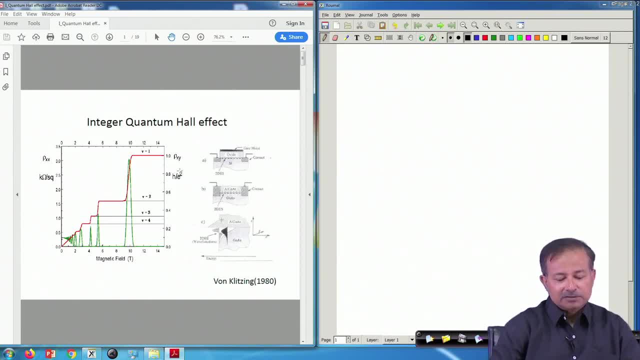 of h to a high precision. then from these quantization, these values of rho xy, you can actually find the value of e square, and that means e. So the application of that was first thought to be in metrology, which is the standard bearers. 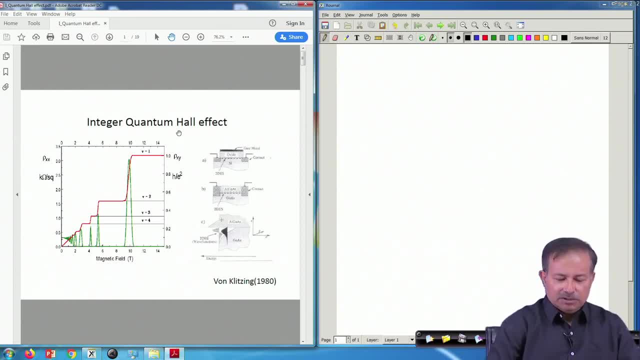 for measurements and units and them and so on. So, like we have in India, we have the National Physical Laboratory keeps our standards, measurement, standard measurements. Similarly the internationally there are agencies which keep the standard And it was thought that this discovery will be very important in finding new ways to fix. 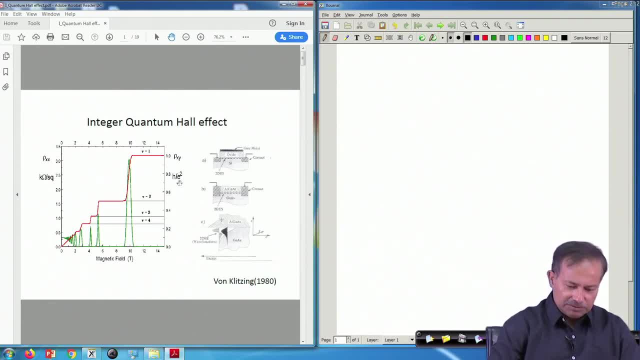 fundamental constants, Now the constants like electric charge and so on. Now, the thing that is interesting here is that the discovery, although it opened up many new avenues for applications and all that, the main attribute of this is fundamental physics, and this physics is so extraordinary. 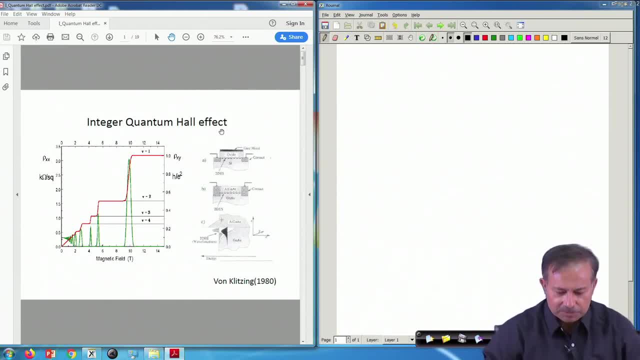 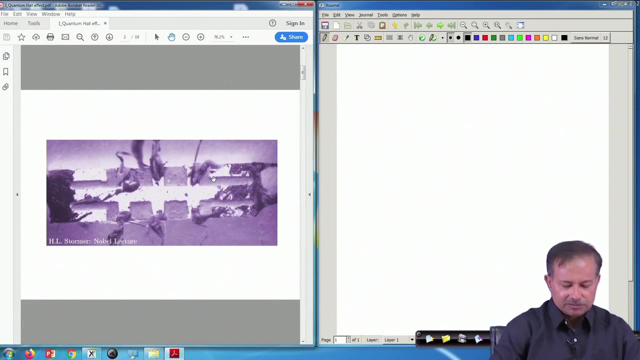 that we should discuss it a bit. ok, Before going there, let me just introduce you to where it happened, and then I will come back to Hall effect and then I will show you how this is done. So this was the original device in which this was done. it is from Stormer's Nobel lecture, So this is how the system worked. 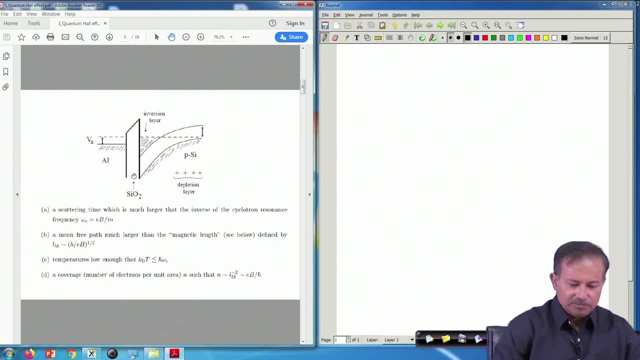 There was a metal which was aluminum. below that there is a silicon dioxide layer and there is a p type silicon after that, And you Confine the electrons in these shaded regions. So, and this shaded region is the inversion layer, and here what has happened is that the you can see that the nature of the potential 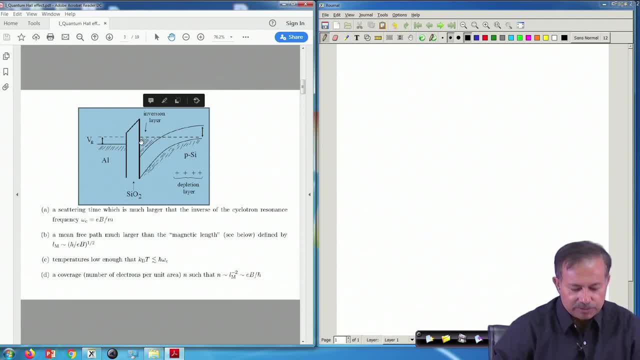 is such that the potential cuts off this electrons movement along this axis, along this direction, and that means the The carriers are confined within the region from this solid line to this, up to this potential. after that it just decays. So there is a confinement of the carriers below this SIO2. 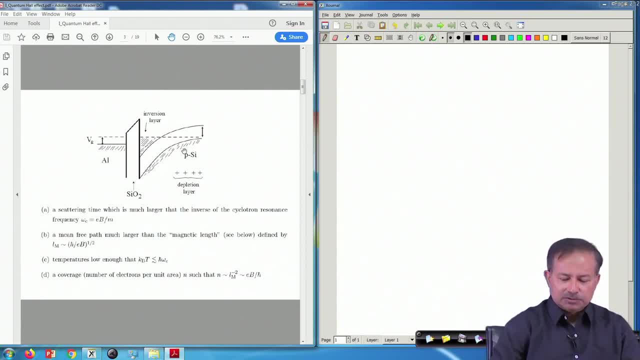 layer within a very narrow region. So- and that region depends on what potential you are applying- I will show you how to. how to do it, and this is physics- is very simple to do this, but, of course, technically it is a challenging. 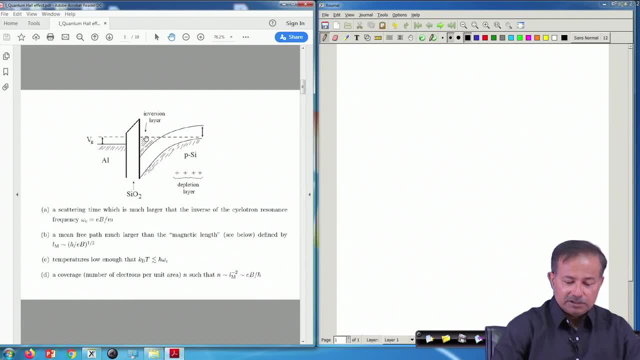 problem to keep the, keep the carriers confined in this region. Now, what are the requirements for this? to show up The system, the where the electron moves, which is this region, must have a very clean sample. So this region must be defect free as much as possible, So that the scattering time must be much higher than the. So the 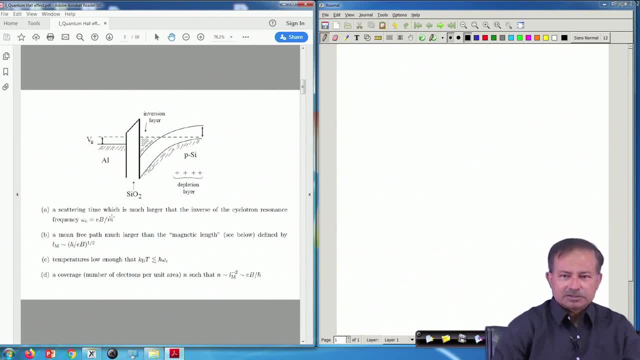 scattering time should be. the relaxation time, which is tau that we have used, must be very, very high, So that there is almost little scattering from defects and so on. And the scale for that is it should be very high, Should be much larger than the resonance frequency. So it is called this cyclotron resonance. 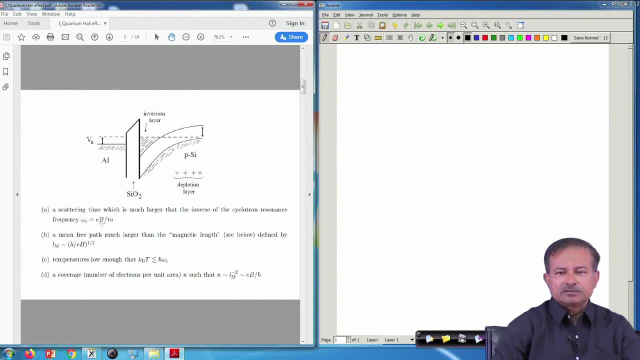 frequency. inverse of that, see cyclotron resonance. frequency is the inverse of cyclotron. Cyclotron resonance has a frequency and that frequency inverse will give you a time, and this time the relaxation time must be much larger than that. Now the mean free path should be very 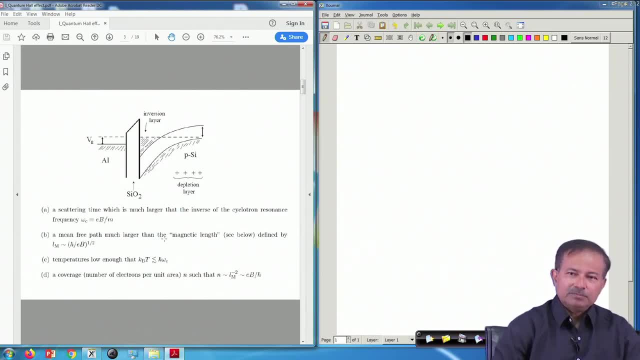 large. The mean free path has to be much larger than another scale in the problem. we will find out what this scale is. it is called the magnetic length, And so the mean free path has to be much larger than this. The temperature has to be very low. Now again, how low it. 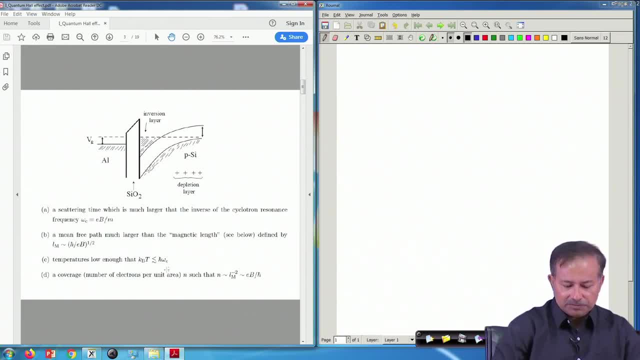 is the means. in a region where h cross omega c is appears to be the gap of the spectrum and the temperature should be such that this energy scale, So the곡 pair corresponding to the temperature, should be lower than h cross omega c. So this is, this is the condition, and, of course, the number of electrons per unit area should. 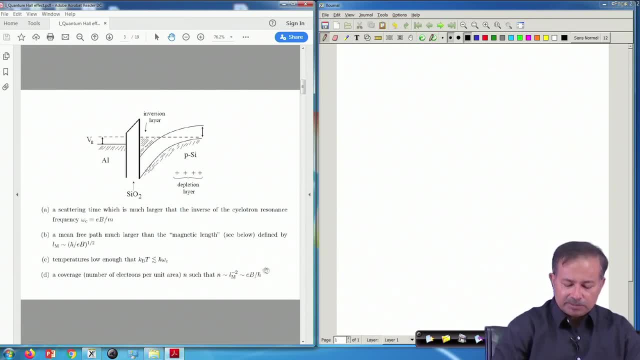 be of the order of E b by h cross. All these numbers, L, m, h cross, omega c and so on, will come out of the Schrodinger equation that we solve for an electron, 2 dimensional electron gas in a perpendicular magnetic field, regular magnetic field. This is actually called the Landau problem. Landau was the first who 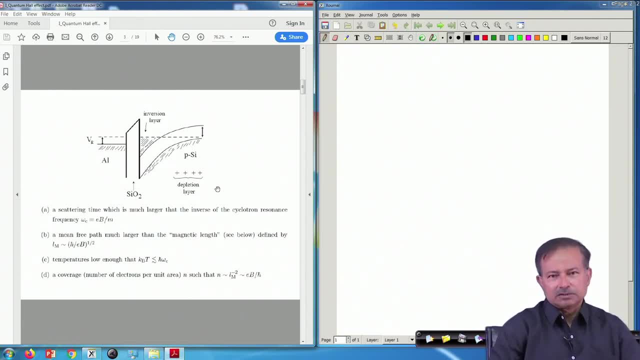 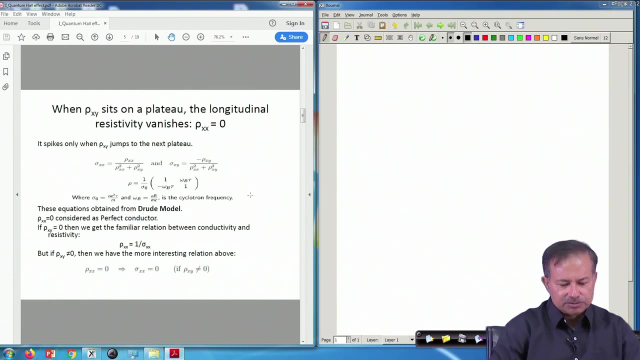 worked out this thing. this calculate worked out this problem and found that the energy levels are quantized. We will do that as we proceed. So I will digress, since I will be using the formulas for Hall effect and all that. I just quickly digress back to Hall effect and let me just show you what we did in Hall effect. 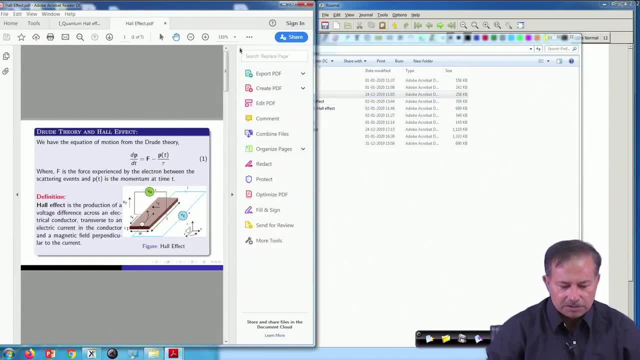 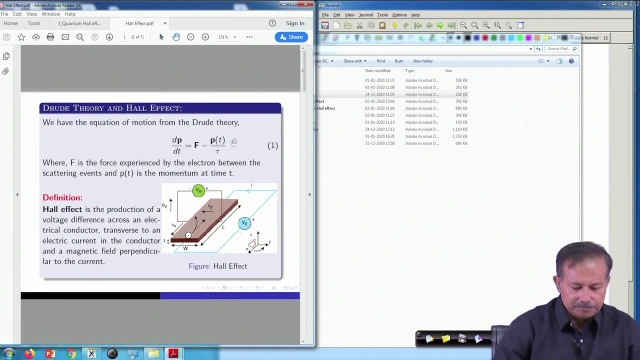 and that is here. Remember your Hall effect diagram. this was the geometry. So you had a sample and a perpendicular magnetic field and then the electrons move Here. of course this is three dimensional, but the there is a sufficient thickness of the of the sample. 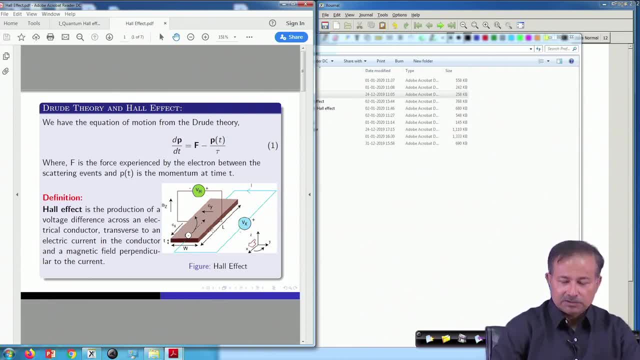 but suppose the thickness of the sample becomes exceedingly small, then you are approaching a two dimensional limit. So, but of course for quantum Hall effect you require more than this. So let us just understand the Hall effect a bit again. This was the geometry. 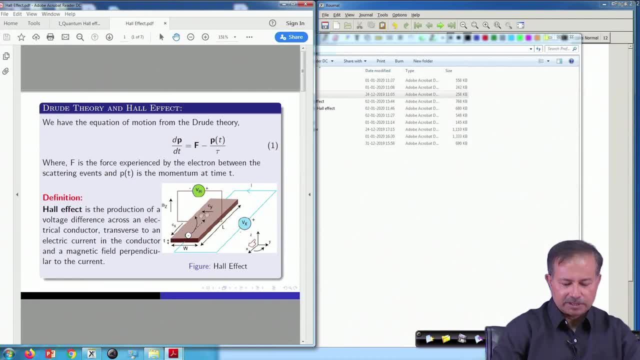 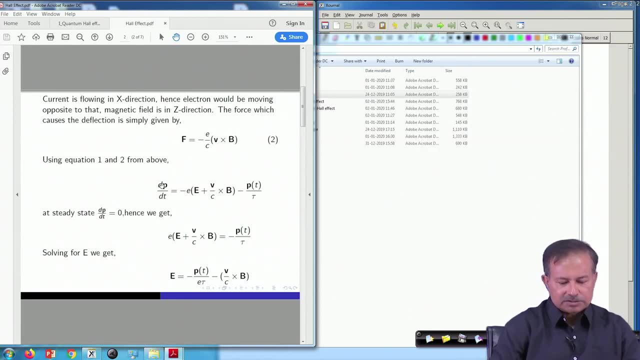 in which we said that there will be a Hall potential developed across this sample. ok, Now what was the equation that we solved? It is simply this, again the. this is the classical Hall effect. I mean simple classical, old Hall effect of the 19th century. So this Drude? 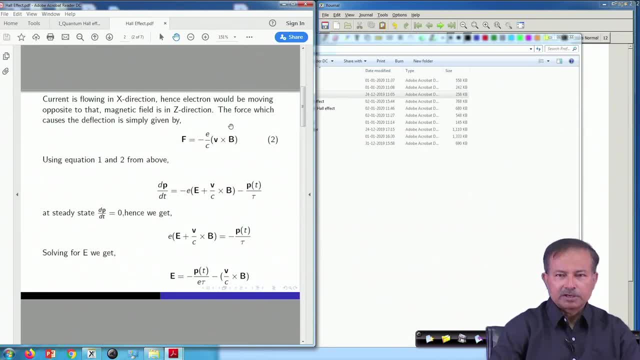 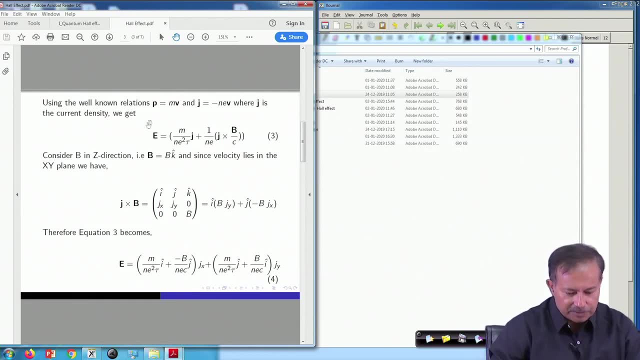 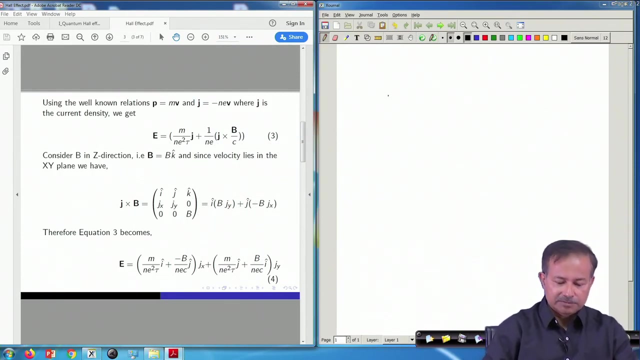 formula is what you used under the force of crossed magnetic and electric field. ok, And we landed up in getting an equation for electric field in terms of the magnetic field, So in terms of the current density, J, x and J, y. So the, so E is, remember, E and J are connected. 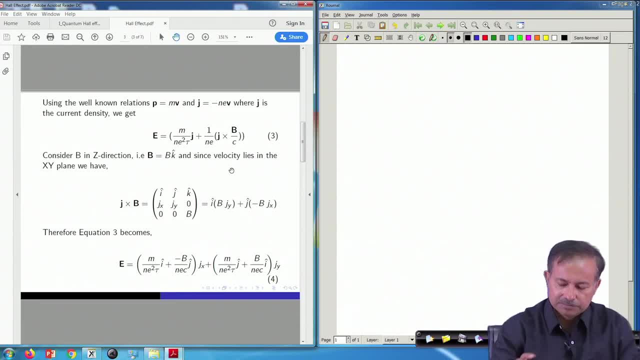 by a, by J, J equal to sigma E, So E equal to rho times J. that is how you can define the rho. So anything that connects E on the left hand side to J on the right hand side, that object is the resistivity. 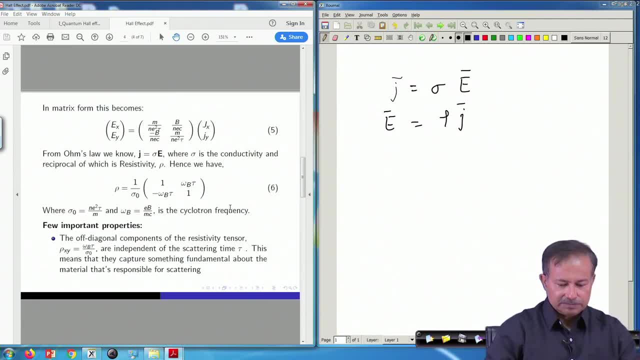 So let us see what comes out of this calculation. So this is what you get. So E, which is E, x, E, y, two components, is a matrix. So E is the matrix time, the J, x and J y. So the rho matrix is therefore remember. 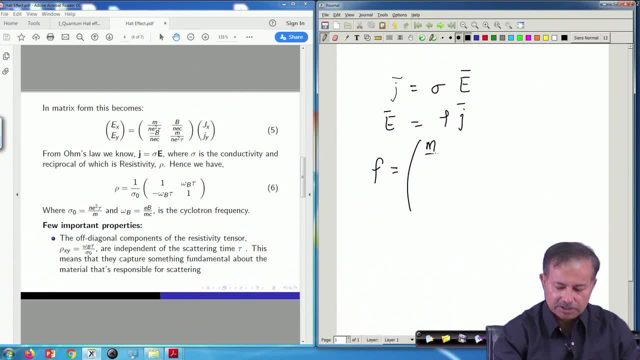 N e square tau by. So let us write it: M by N e square tau. tau is the relaxation time. B by N e c, B by N e C and M by N e square tau. So that is your rho. Now, what has been done in equation? 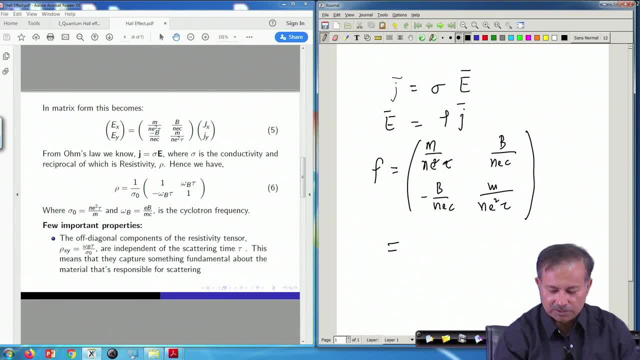 6 is that just M by N e square tau has been taken out as, and then you can write this as 1 by sigma naught. Remember our Drude formula: sigma naught used to be N e square tau by M. ok, So that is so. that is why this is 1 by sigma naught. and if you do that, then 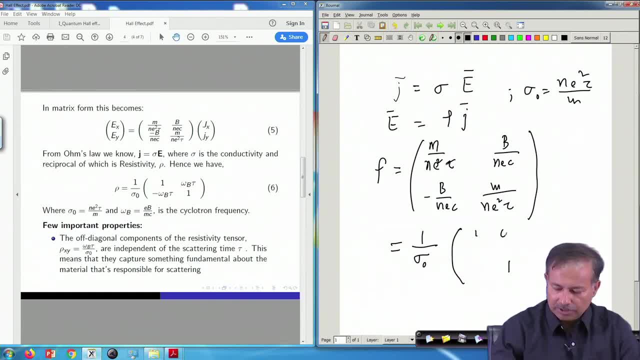 you will get 1, 1 omega B into tau, minus omega B into tau. So rho xx equal to 1 by sigma naught, 1 by sigma naught, and rho xy equal to omega B, tau equal to minus rho xy, rho yx, ok, So. 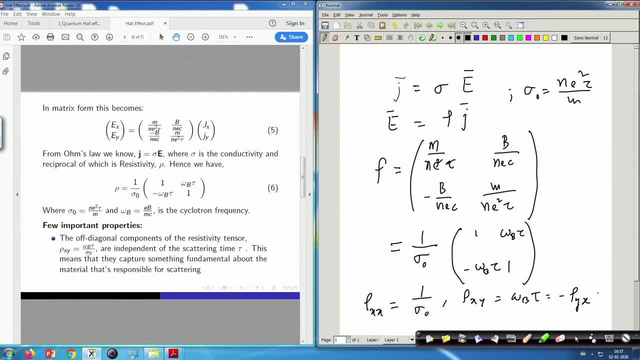 this is the So this is the formula that we obtain for resistivity. So resistivity is no longer a scalar quantity, it is a matrix. and that matrix couples connects the current density, which is two component here, J x and J y- to electric field, which also has two components. 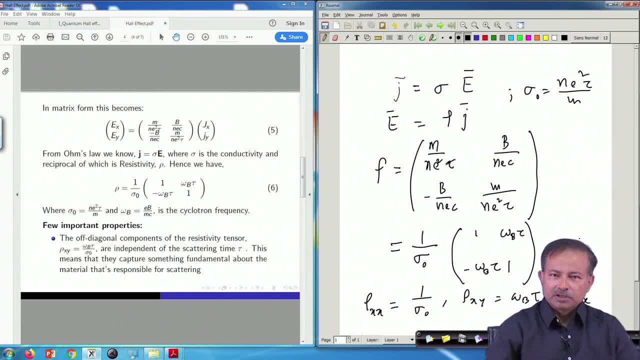 One component is the applied one and the other one is developing because of the modulation of the electrons away from the direction of magnet, the direction of electric field due to the magnetic field. So that is E, y, the transverse field that generates. ok. 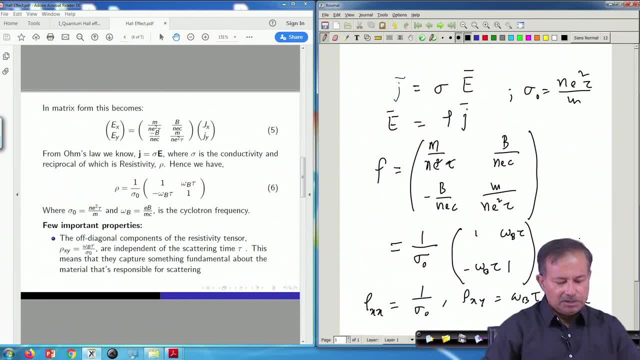 So this was what we did. The one thing that you should notice is that the- this is the ok. So rho x, y is omega B tau divided by sigma naught. Now this sigma naught has a tau in it, So this will cancel the tau that appears here right. So that means the off diagonal. 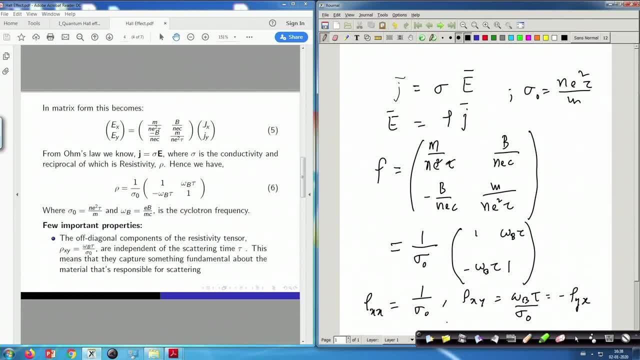 resistivity is independent of the scattering time. ok, So that is interesting, 18.56.. this is then. this then becomes independent of the property of the system, right, Because omega B is equal to E, b by m. c c is a fundamental constant, m is the mass of the carrier, and 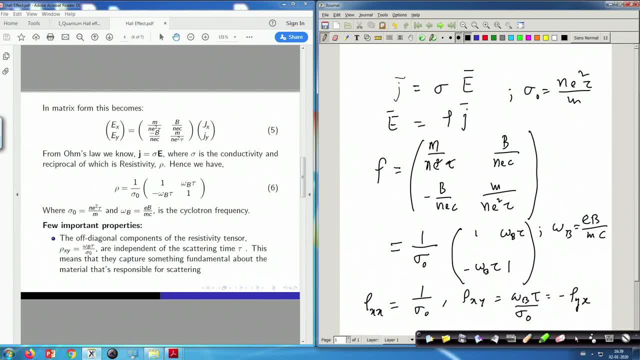 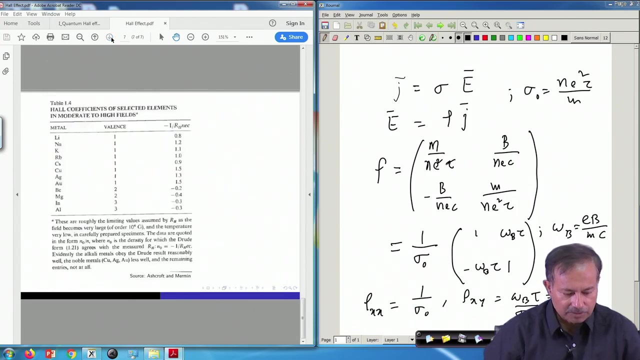 B and E are. B is applied externally, E is also a fundamental constant charge of an electron. So the, this quantity, rho, x, y, becomes a fundamental kind of quantity which does not depend on material properties. So this was the classical Hall picture that we got. So let us now close. 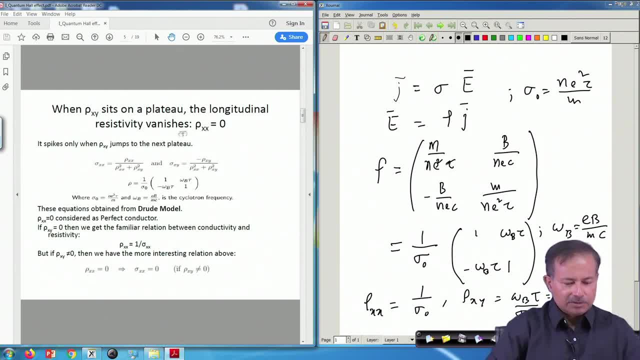 this and we go back Back to the quantum calculation, which is, which is? which actually is very similar to the classical calculation. up to this far, we will do the same thing as you did in classical mechanics. This formula works even in quantum mechanics, So there is nothing quantum about this formula. 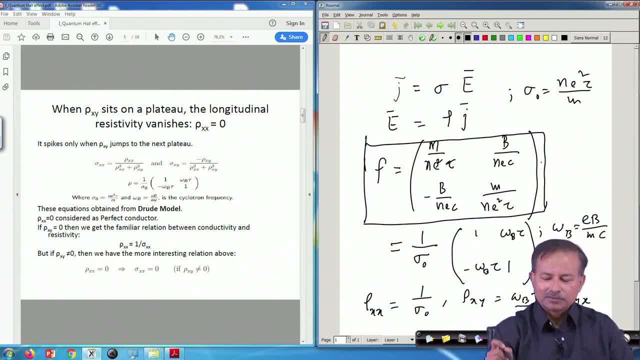 The thing that is going to affect in quantum mechanics, Going to be affected is this N, The N in Q m is the culprit that gives us the, the, all the properties that a quantum Hall system that I showed in the beginning, that quantum Hall system has comes from the quantization of these energy levels and therefore the 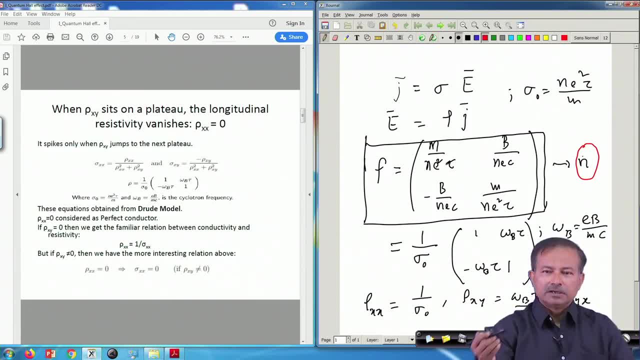 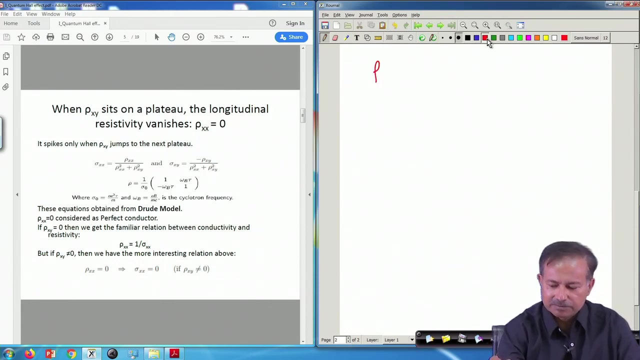 N Type is a. I can show that there is a. n is a multiple of some number times an integer. So let us proceed. there is a interesting caveat that is here. remember that if you have a scalar relationship, remember sigma x, sigma rho xx, equal to 1 by sigma xx. If you did. 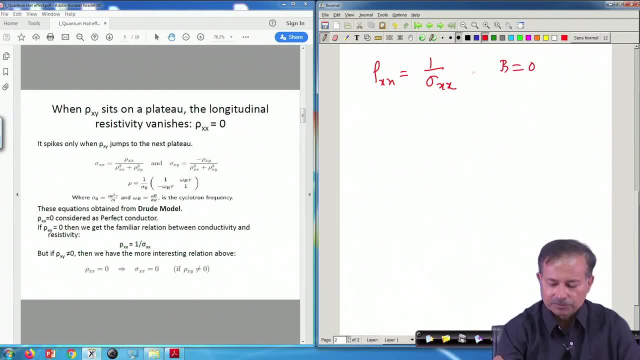 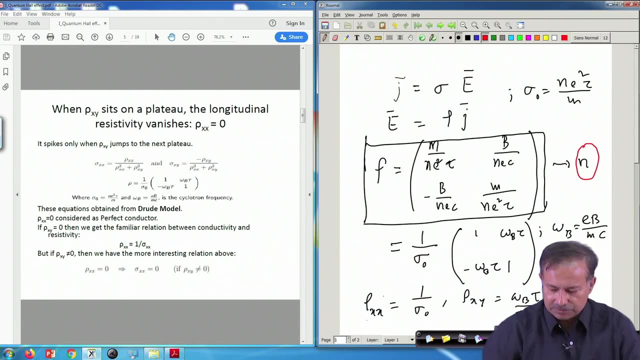 not have b equal to 0. ok, if you had b equal to 0, then this relation goes through. So then you remember. this is one I am saying. suppose there is no off-diagonal component, b by any c is then 0 and then of. 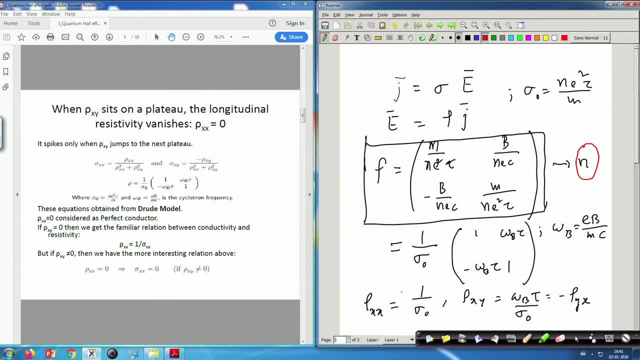 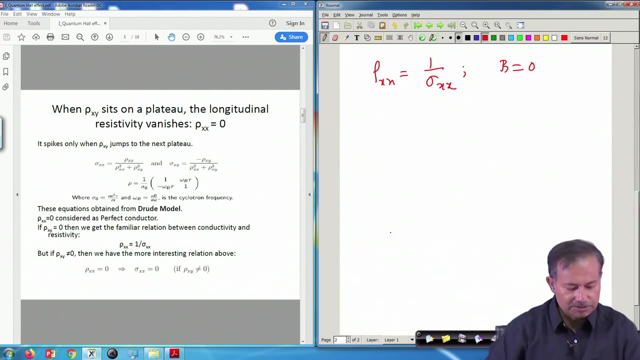 course. then rho xx goes through as 1 by sigma, or that goes through even here, but that is now an. there is no rho xy, then ok, Whereas what is interesting here is that when b is non-zero, that means your rho xy is non-zero, xy not equal to 0, which is b not. 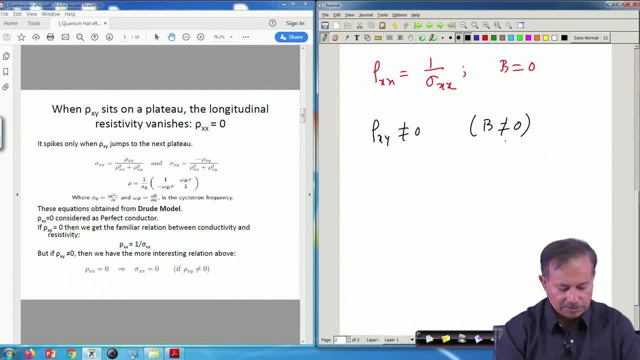 equal to 0, then you see what happens. then you have rho xx equal to 0 implies rho sigma xx equal to 0 as well. This is really interesting here. for example, in the top relation for b equal to 0, if sigma, if rho xx goes to 0, sigma xx will be, will have infinite conductivity, Whereas here: 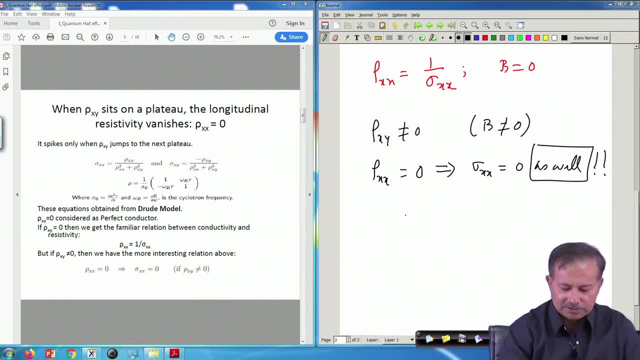 and the reason is very simple, that if you look at this expression for sigma xx, it is just the, So you just invert the matrix and then you will get rho xx by rho xx square, plus rho xy square, and sigma xy equal to minus rho xy by rho. this, the denominator, comes from. 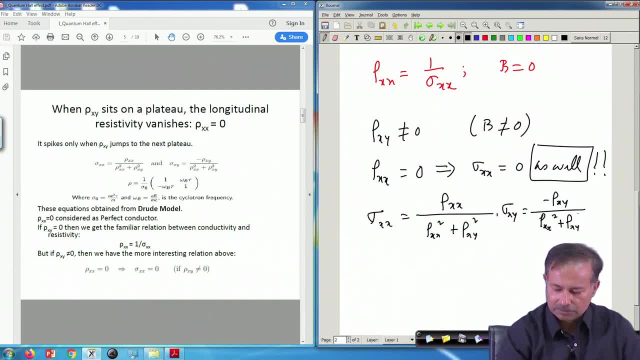 the determinant plus rho xy square. So that is what exactly what this says. this one says that: So you set rho xx equal to 0, then sigma xx also goes to 0, because sigma xy is non-zero, sigma x, rho xx is 0.. So the denominator is finite where the numerator becomes 0.. So 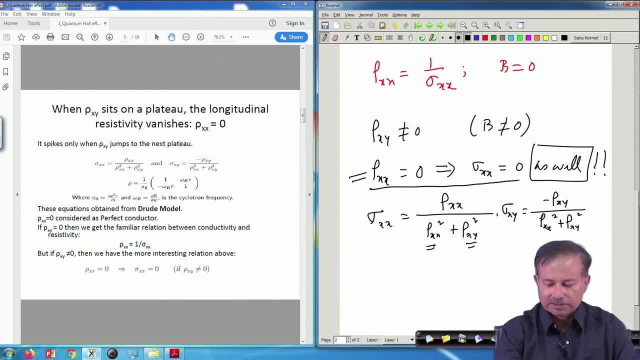 this implies that rho xx and sigma xx can simultaneously be 0. So this is really interesting. So it is very remarkable. this says that in presence of a magnetic field, you have a situation where both diagonal conductivity and which is longitudinal conductivity and the longitudinal 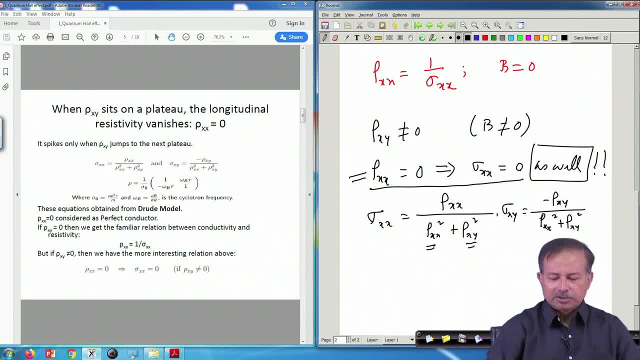 resistivity can vanish, together can become 0. If one becomes 0, the other will become 0. So that is remarkable. and when does that happen? Well, it we will see when the that happens. That happens because, again, the sigma rho xx vanishes, because there is no dissipation. 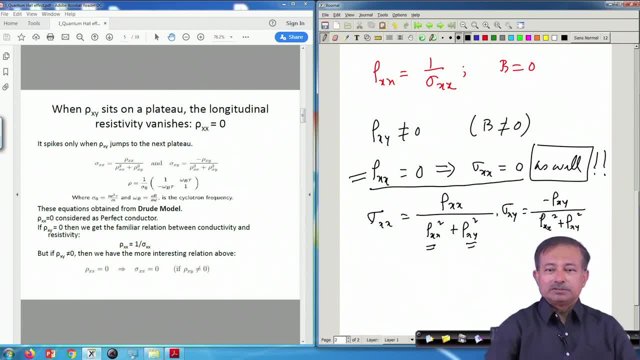 in the system It is. there is absolutely no dissipation in this in this system, whereas sigma xx going to 0 means there is no conductivity, which means that there is a gap in the spectrum. So these two things come from two different sources, but it is remarkable that compared. 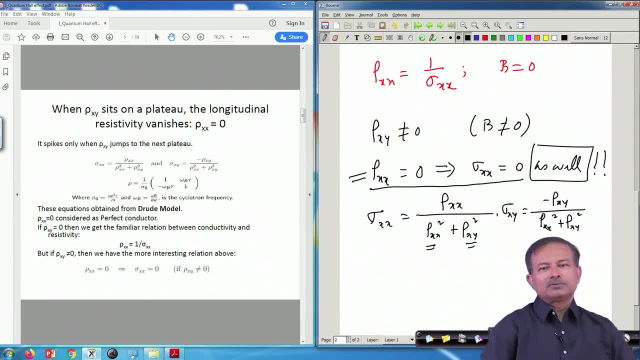 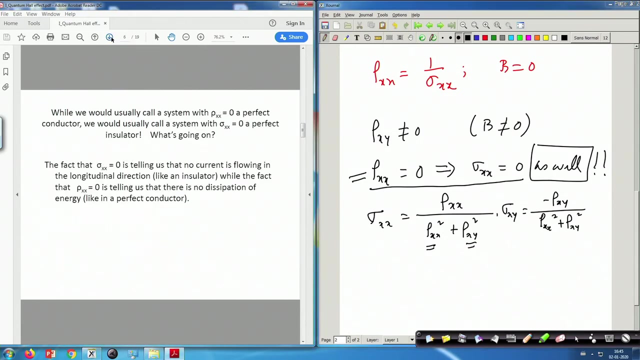 to a single, compared to a situation where you do not have a magnetic field which makes the resistivity or conductivity as tensor. you have to rethink about your physics in a way which is non-trivial already, even at the level of classical mechanics. ok, So let us now go forward and see what we So. this is what you say, the in fact that 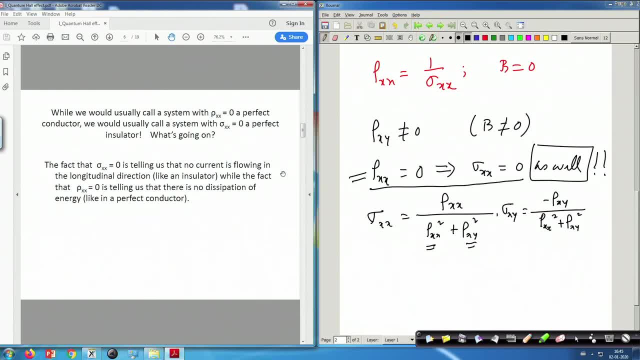 sigma xx, equal to 0, is telling us that no current is flowing in the longitudinal direction like an insulator, which means there is a gap in the spectrum, Whereas the rho xx, equal to 0, is telling us that there is no dissipation of energy, like a perfect conductor. So it 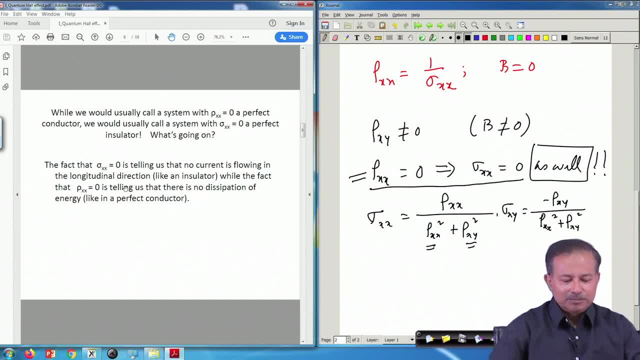 is a perfect conduct: No dissipation, but it is a. it is has. is sigma xx equal to 0, because there is a gap in the spectrum which is like an insulator. So that is, that is really remarkable. and that happens without any introduction to quantum mechanics or anything. it is just because of